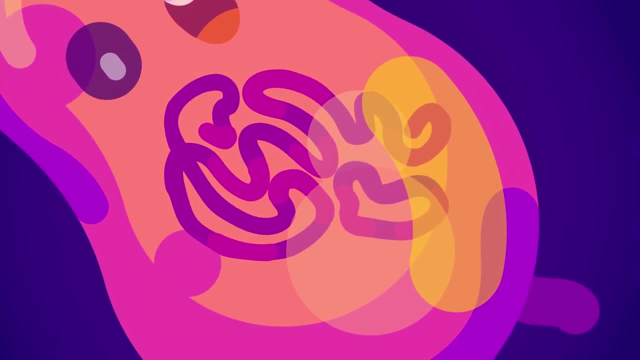 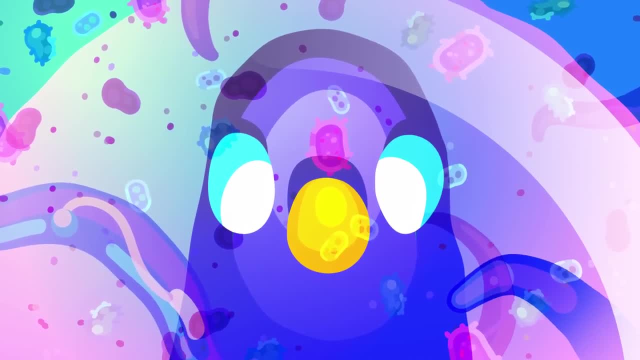 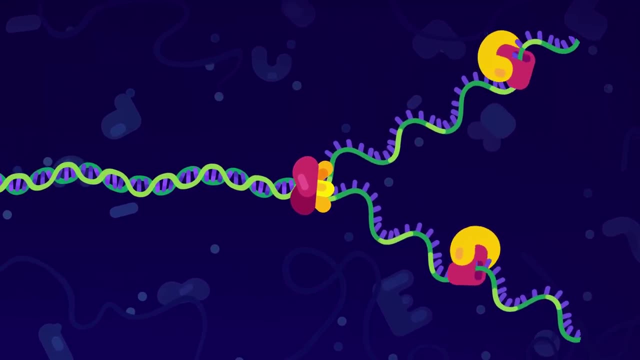 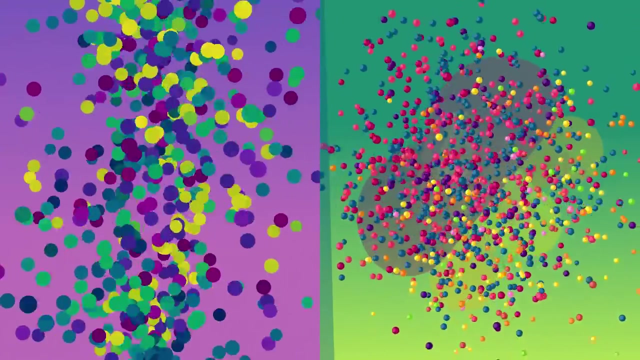 How dead things with no genome become living things with genomes is one of the biggest riddles of science. Simplifying a lot, the problem is that to have a functioning genome you need proteins and to make those proteins you need a functioning genome. Both proteins and genomes are super-long molecules made of pretty complex blocks. 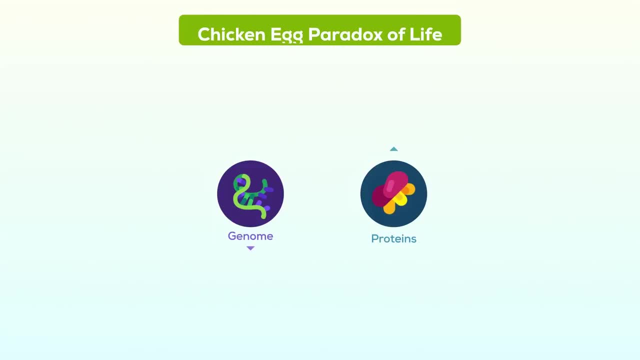 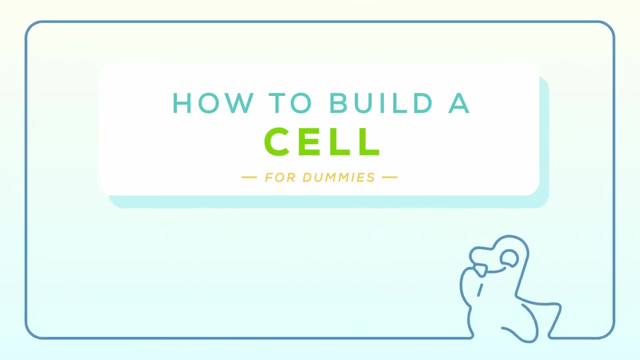 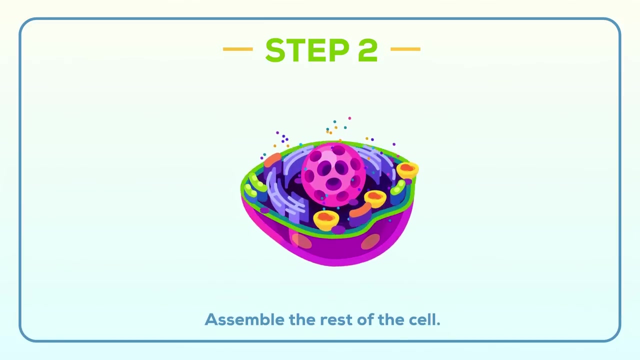 that are extremely difficult to assemble by chance. It's a chicken-egg paradox with several chickens and eggs. Once you have a finished cell, the whole system works efficiently. But starting from simple dead stuff and reaching that level of sophistication by pure chance should require an amazing amount of time for trial and error. 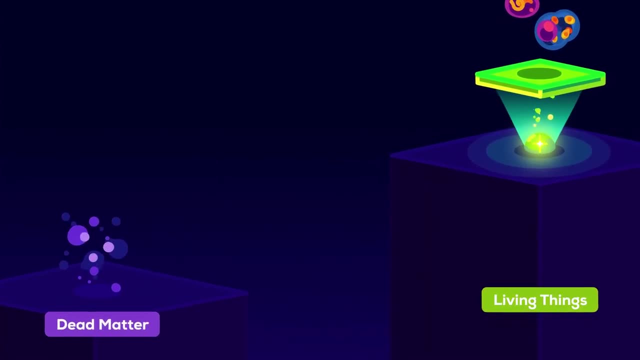 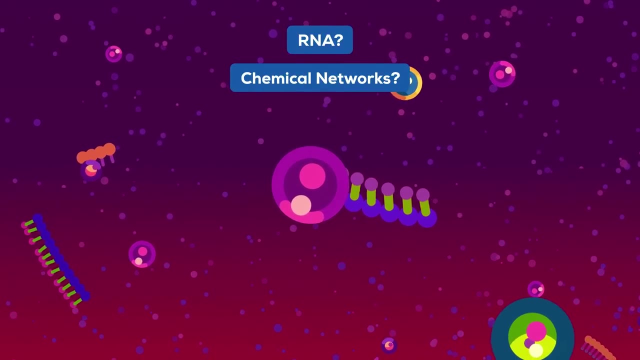 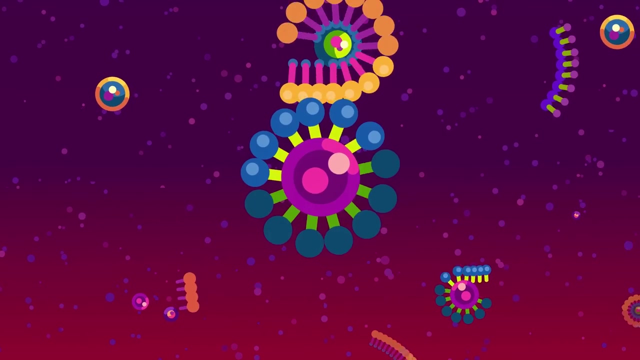 So how did the first living things manage to cross that gap in just a few hundred million years? Most theories about the origin of life try to explain that gap by theorizing how some primitive soup of prebiotic molecules could have efficiently produced the first self-replicating entities. 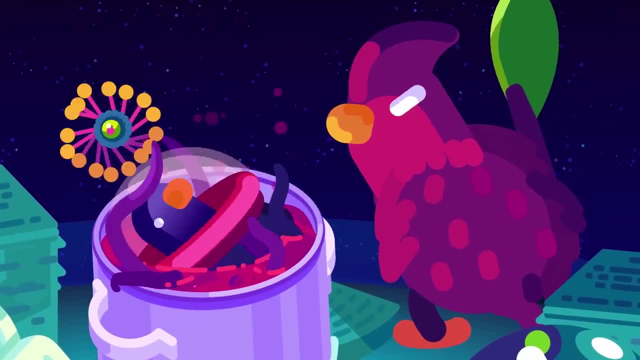 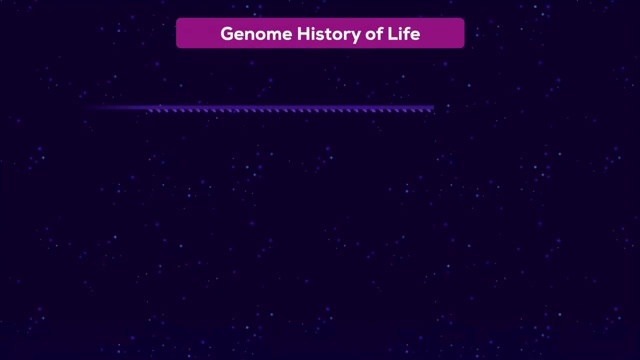 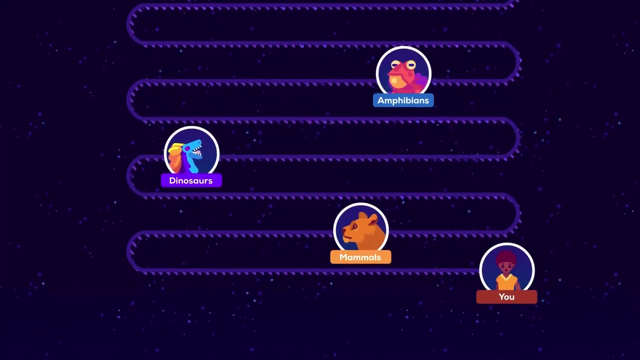 But we still don't know how exactly this would have worked. Maybe we need to think backwards. The Clock of Evolution, Think of genomes as a book telling the history of life. As time passed and life evolved, more characters were introduced: Amoeba, fish, amphibians, dinosaurs. 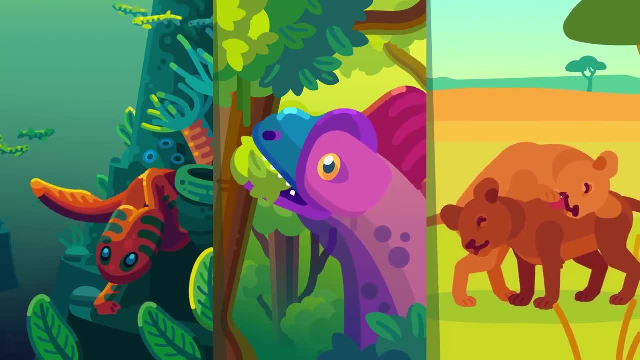 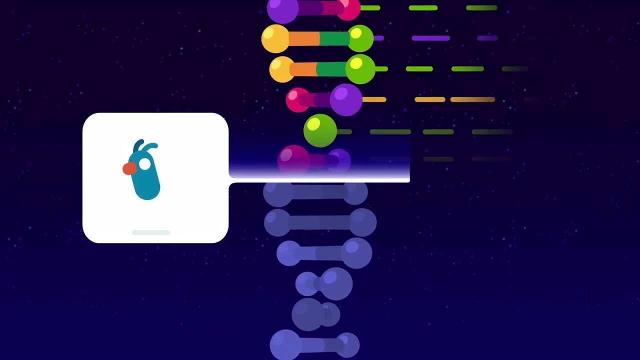 And mammals. Over billions of years, the story of life got more and more complex. A genome can be viewed as a long string of letters with biological instructions And from microbes. to us today, functional genomes seem to have been increasing in size at a fairly constant rate. 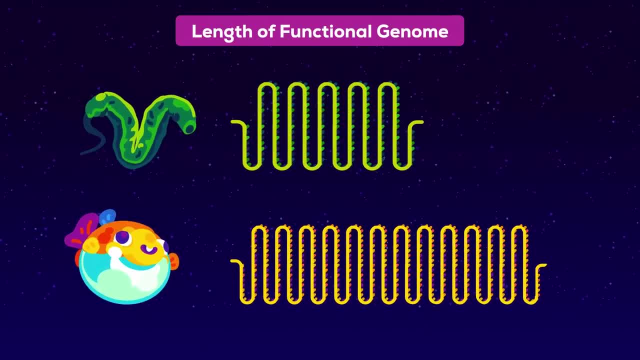 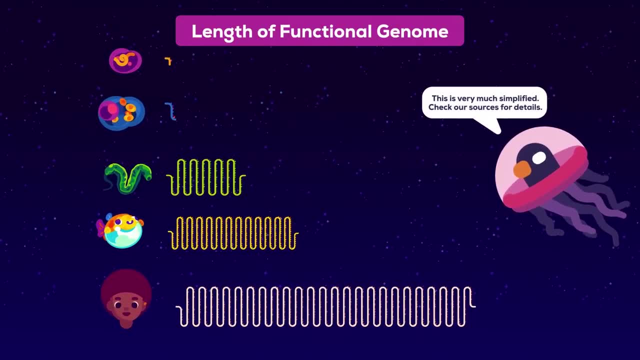 The functional genome of fish is more than twice that of worms, Our functional genome is about twice bigger than that of fish, and so on. It is a bit more complicated, but for now let's run with this. When we put all these clues together, 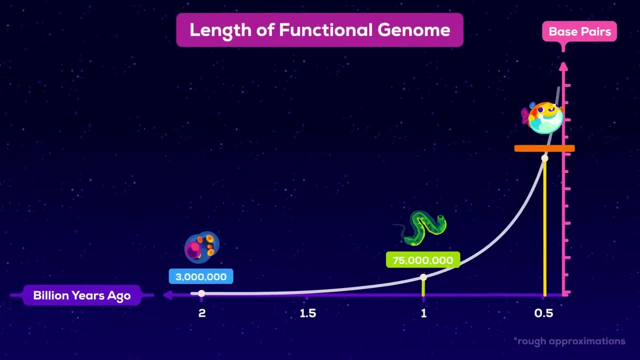 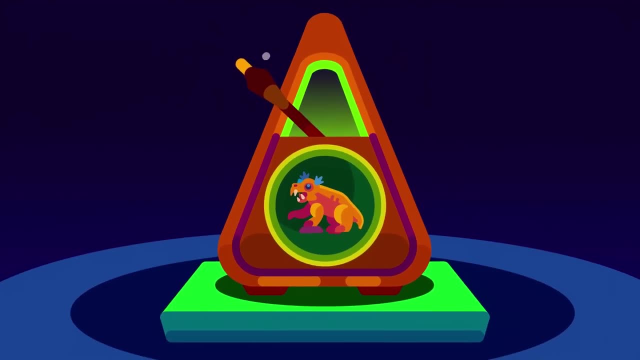 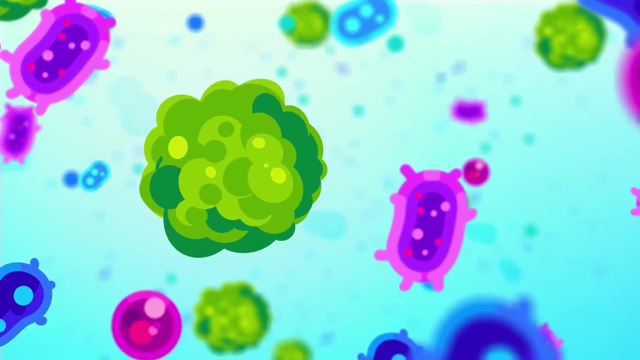 it seems that genomes have been doubling in size on average every 350 million years or so, As if evolution had been following an exponential inner clock. But it gets even stranger: The very first microbes that emerged on Earth, even if they look simple. 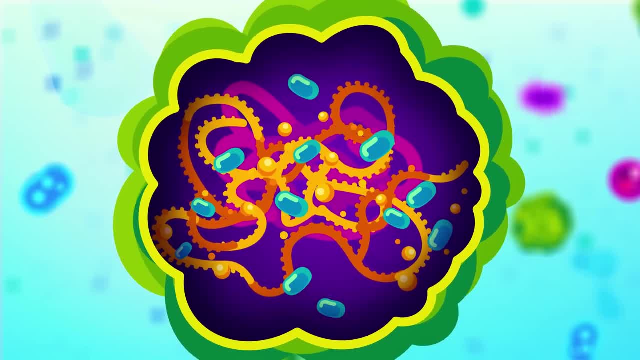 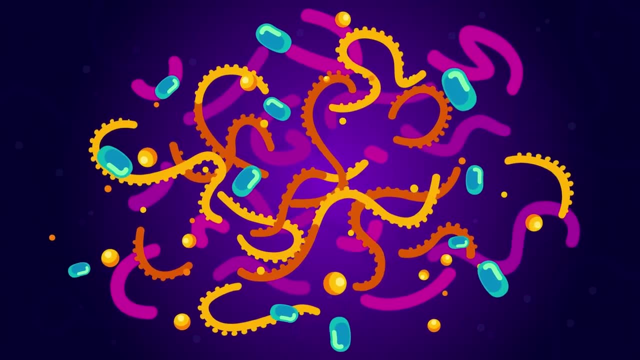 already seemed to have had pretty long and complex genomes. But how could life have achieved that level of complexity in such a short time? There may be an interesting way to solve this riddle. We just take our exponential clock and extrapolate it back in time. 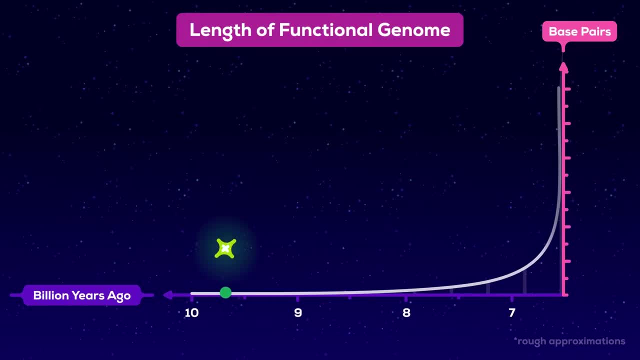 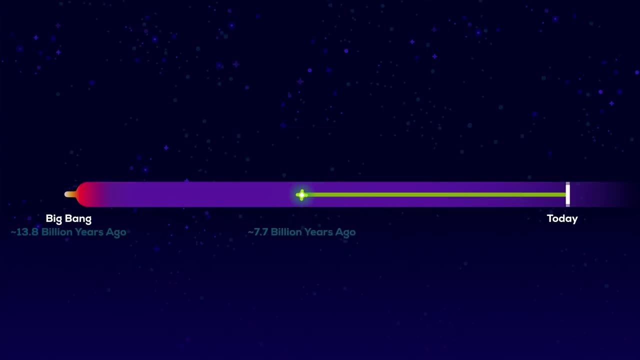 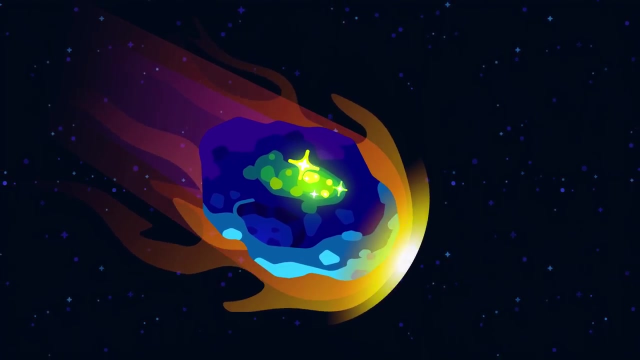 to the simplest conceivable life form, Something equivalent to a being with a genome containing just a few letters. But if we do that, we end up 10 billion years in the past, More than twice the age of Earth, Which means if life actually evolved like this, it didn't start here, but somewhere out there in space. 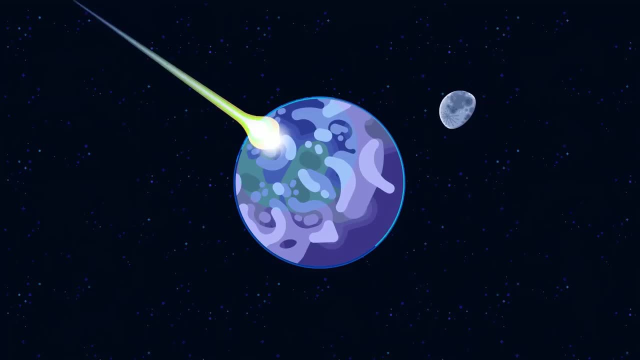 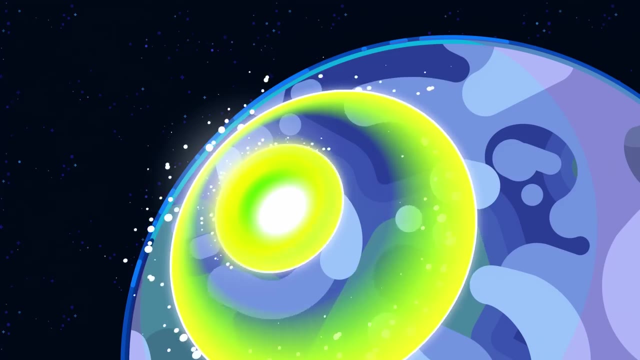 This would explain why life started to thrive so quickly on our young planet. If it was already present in space like a seed, it just needed water and warm temperatures to wake up and go on evolving. And it would also explain the high degree of sophistication of the first life forms on Earth. 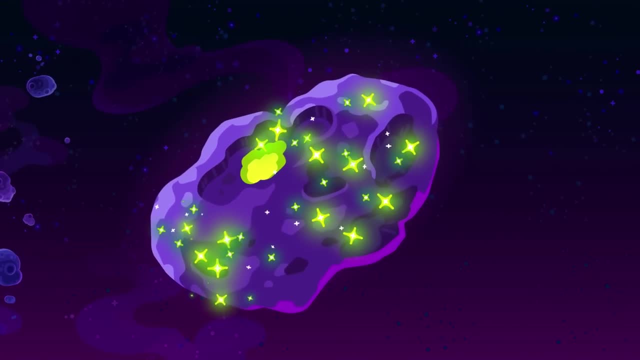 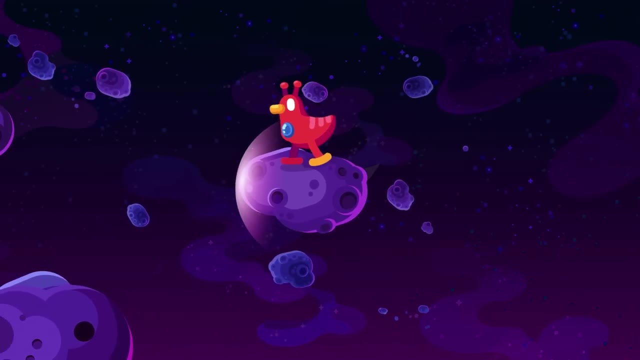 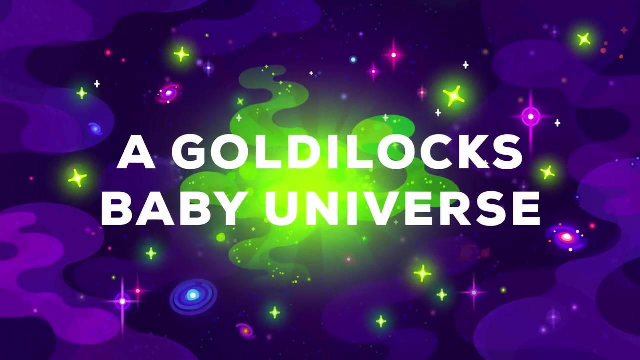 They could have been complex already, because they might have been evolving for billions of years somewhere else in the universe. But could life really be that old? Maybe, yes, Actually, life could have started shortly after the universe itself was born. A Goldilocks Baby Universe. 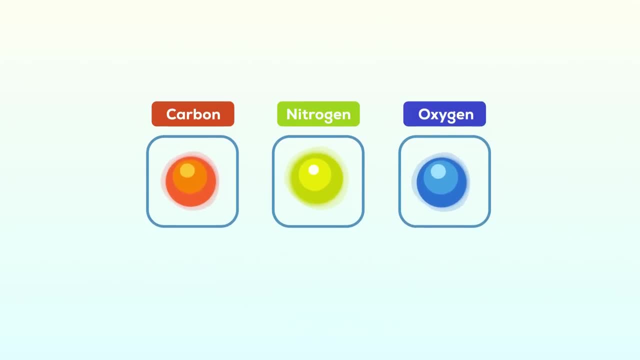 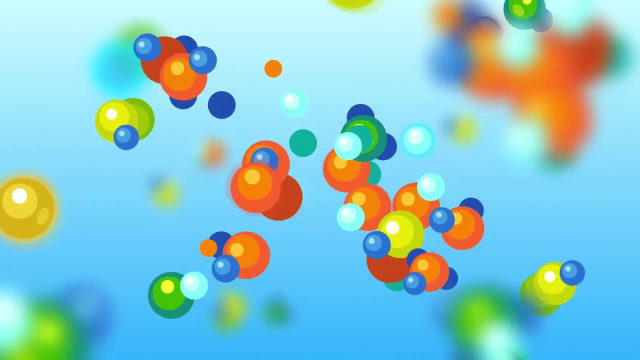 At its most basic level, life needs two things: The right chemical elements to form complex molecules and a liquid medium like water in which those molecules can move and interact. The liquid medium needs to stay warm enough to remain well liquid. 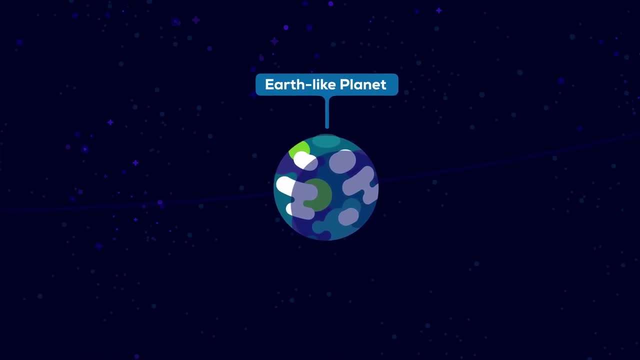 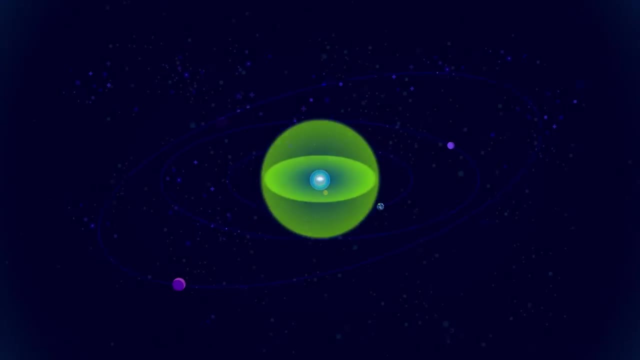 So when we search for life in space, we focus on Earth-like planets at just the right distance from their star. The universe has been meant to be warm enough to sustain liquid water, But there was actually a time when almost all of the universe might have been habitable. 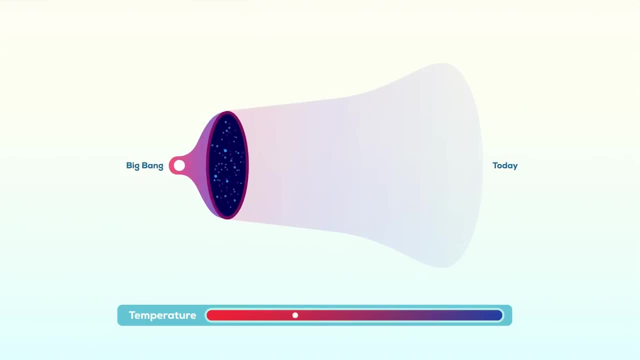 Right after the Big Bang, the universe was extremely hot, But as the cosmos expanded, it cooled, And between about 10 and 17 million years after the Big Bang, when the universe was a thousand times younger than today, it was between 100°C and 0°C, the temperature at which water is liquid. 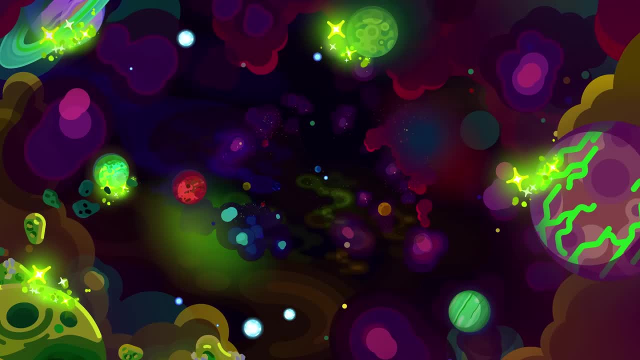 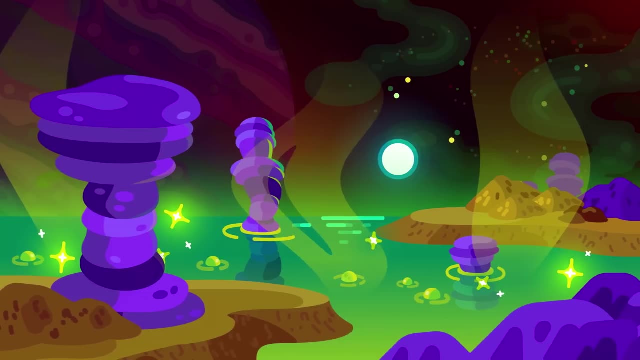 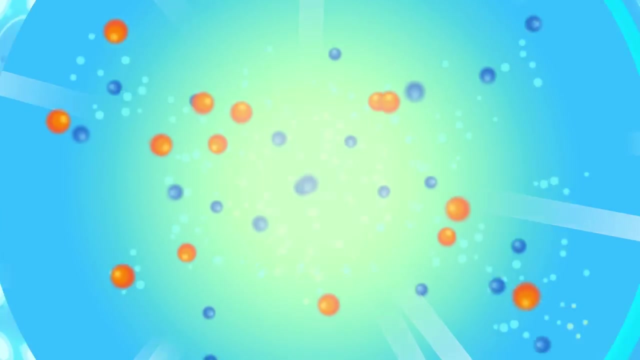 of time, more than 13.7 billion years ago, the whole universe, absolutely every inch of it, had the right temperature to support life. Of course, the right temperature alone is not enough for life. We also need chemical elements like carbon and oxygen, which are forged in the cores of stars. But were there stars in super early cosmic times? Maybe, yes. in regions of the universe where matter was especially dense, Such stars would have been very massive and gone supernova in just three million years, seeding the baby universe with the chemical elements. 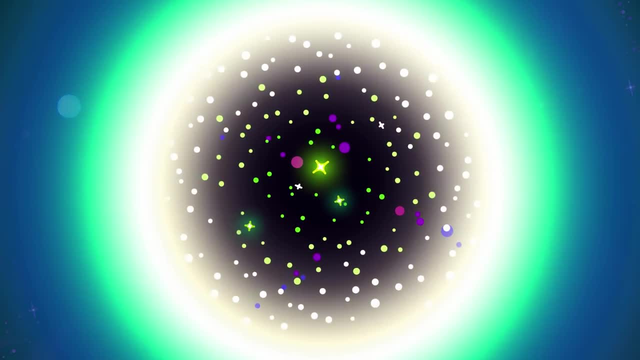 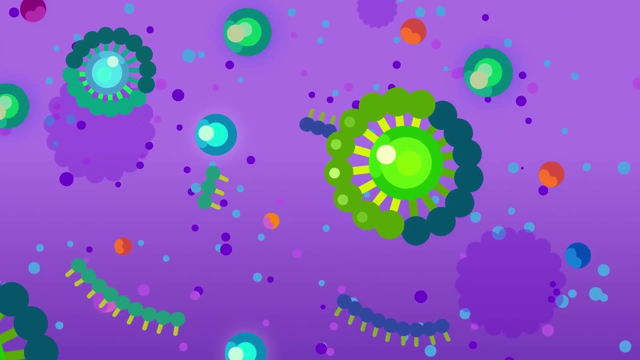 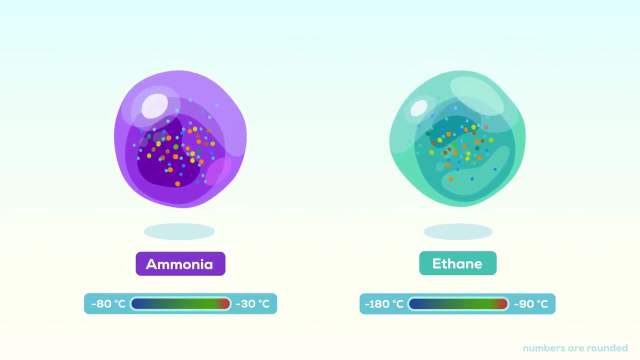 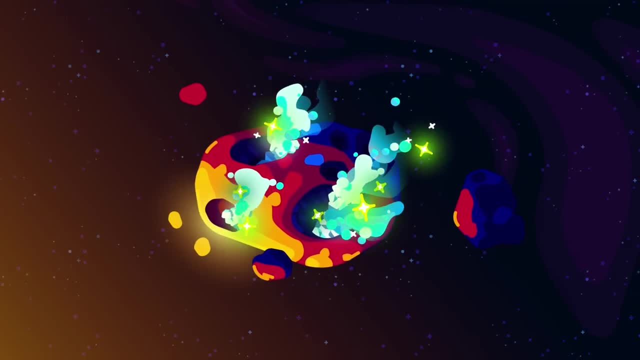 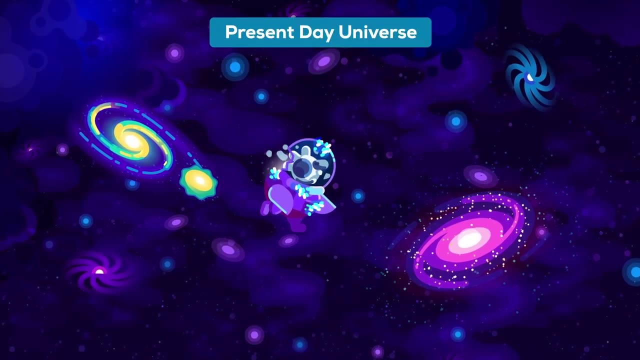 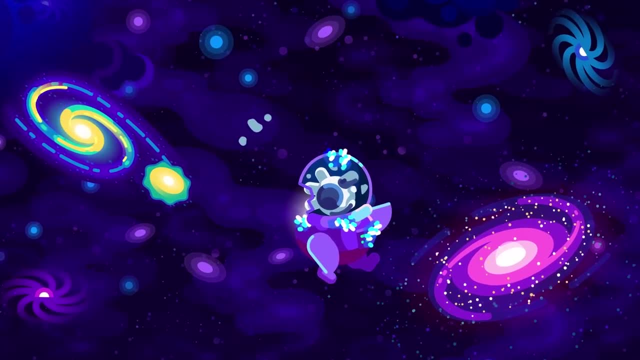 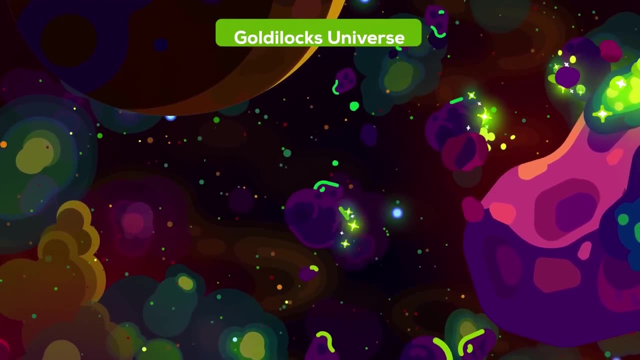 is that, while the universe today is extremely deadly and hostile, back then the conditions for life might have been basically everywhere For a period that may have lasted several dozen million years. primordial life might have been able to emerge on any rock, even between the stars. Sowing the universe with the sea and the ocean, the universe would have been able to emerge on any rock, even between the stars. Sowing the universe with the sea and the ocean, the universe would have been able to emerge on any rock, even between the stars. seeds of what, billions of years later, would become bacteria, trilobites, dinosaurs and, finally, us. At some point, the universe cooled down below the right temperature for life to thrive, but some of those ancestral lifeforms may have continued to exist in the internal warmth of. 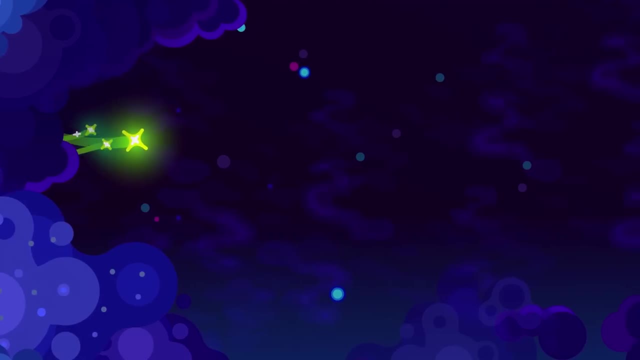 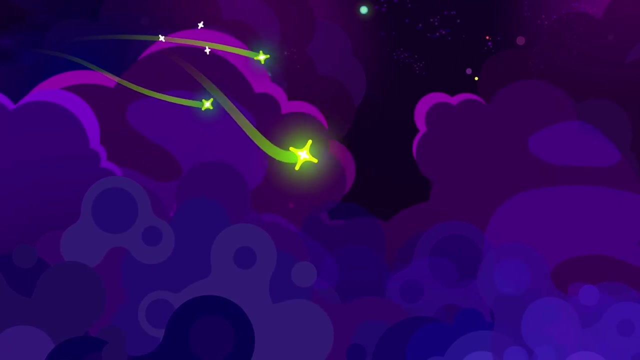 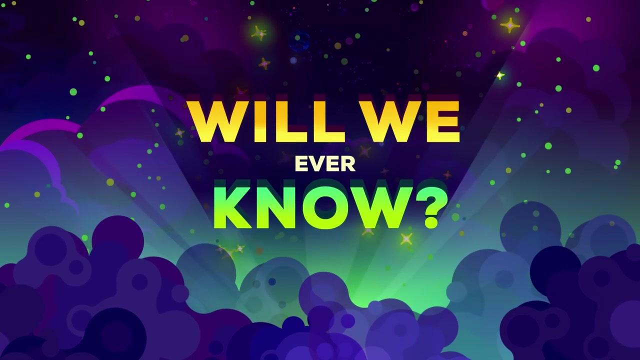 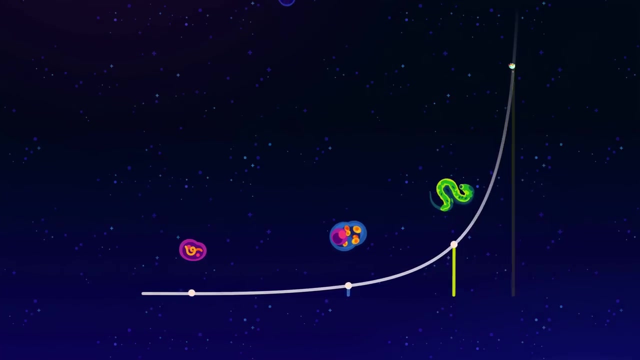 the first planets, frozen in asteroids or hibernating in cosmic dust, tiny seeds roaming the cosmos waiting for new hospitable places to continue evolving. If they did, life now might be everywhere in the universe. Will we ever know? All this makes for a nice story, And while both the habitability of the baby universe and our exponential clock of life are reasonable ideas, they're still speculative.